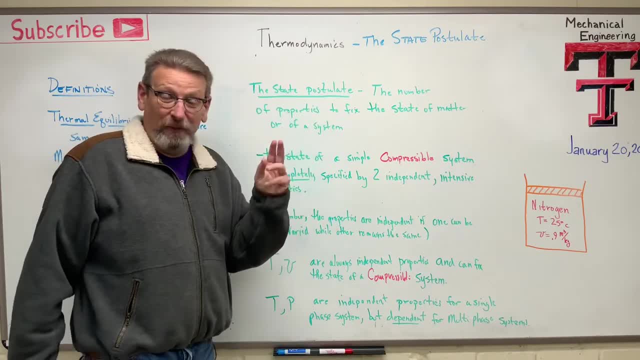 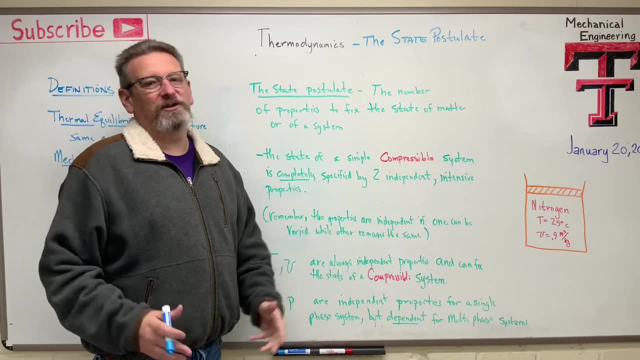 Okay, hello my friends and welcome back to. you're with me for the Thermodynamics video number three. You're doing good. Here we go. I know today is going to be more definitions. Y'all are ready to start working some problems. We're kind of laying the groundwork here with definitions. 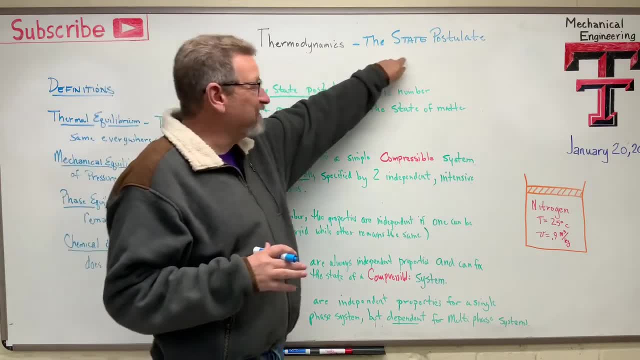 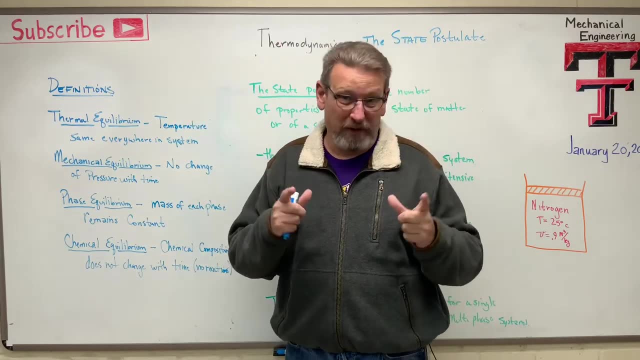 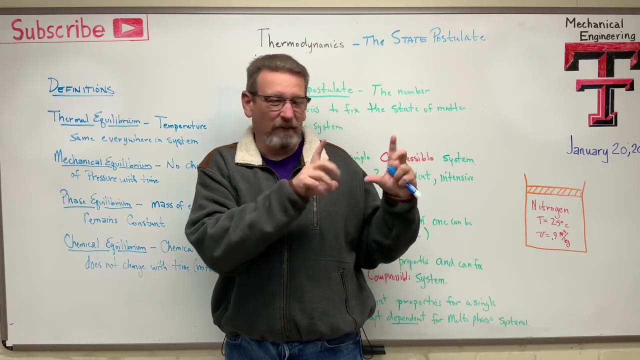 before we get started. So today we're going to be talking about the state postulate. What in the world? okay, Let's start off talking about equilibrium. okay, When we say that the state of matter or the system is in equilibrium, it's in global equilibrium. what does that mean? Well, 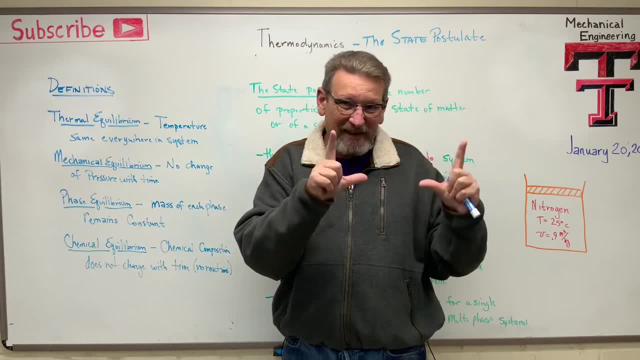 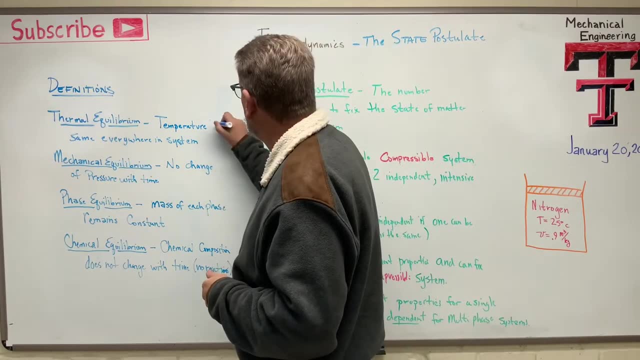 all of these kind of conditions have to be met for that to be in equilibrium. okay, So, number one, you have to have thermal equilibrium, which means this: right, If I have a system, I don't know it has some kind of gas or something in it. right, If I have a molecule over here that's at 50. 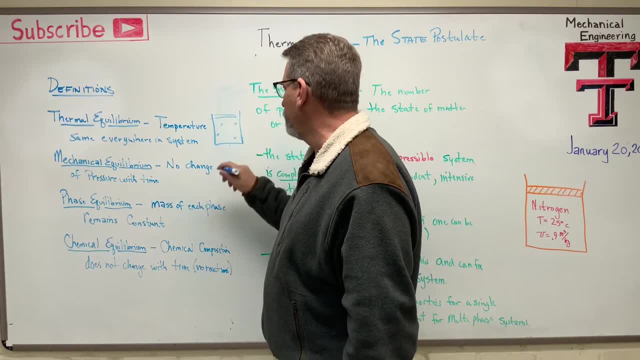 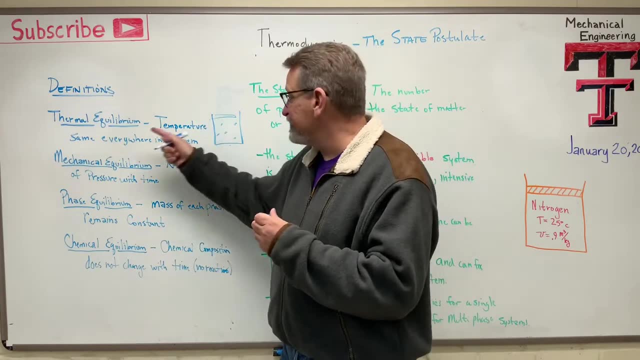 degrees: one over here that's at 30,, one over here is 20, and this guy's at 40, and there's one at 37, right, Then, that's not in thermal equilibrium. So, thermal equilibrium, the temperature is the same. 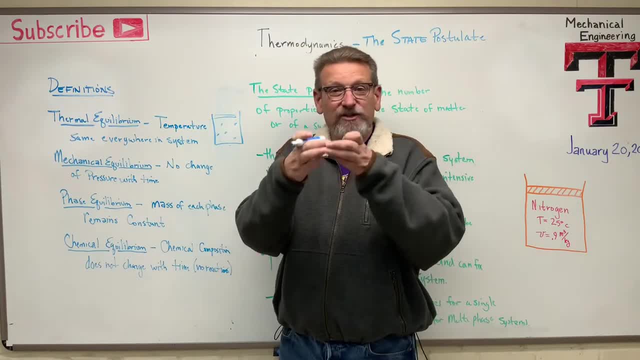 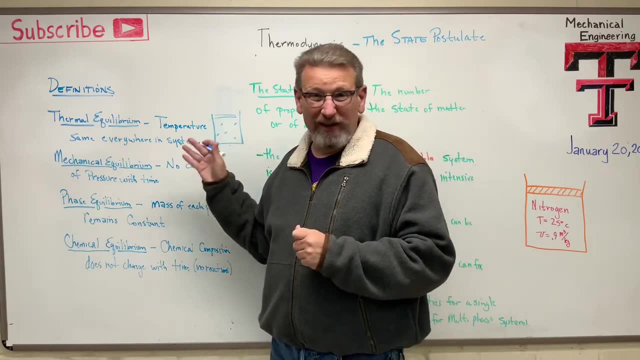 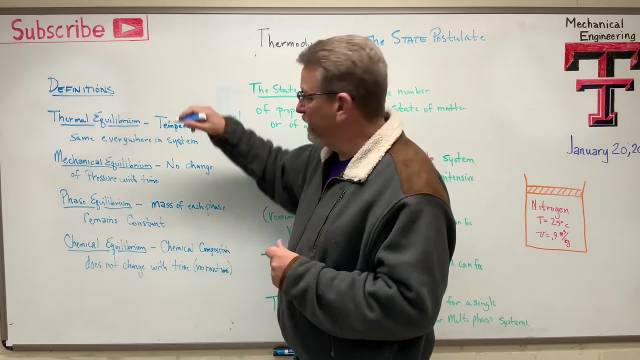 everywhere in the system. So it's been sitting there, it's all normalized, it's all equalized. everything is the same, every molecule is the same throughout the system. Now we have thermal equilibrium, There's mechanical equilibrium- okay, So there's no change in pressure with time. 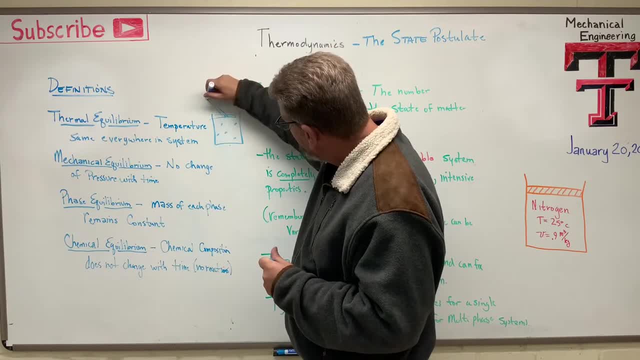 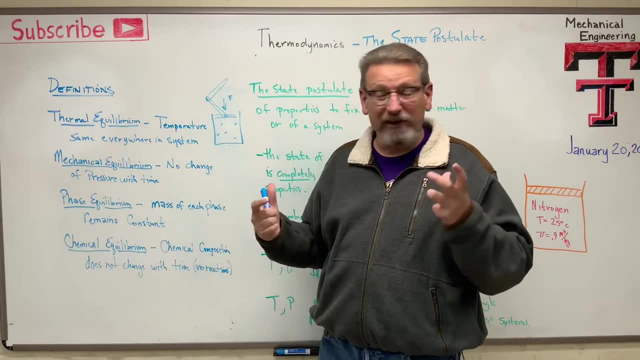 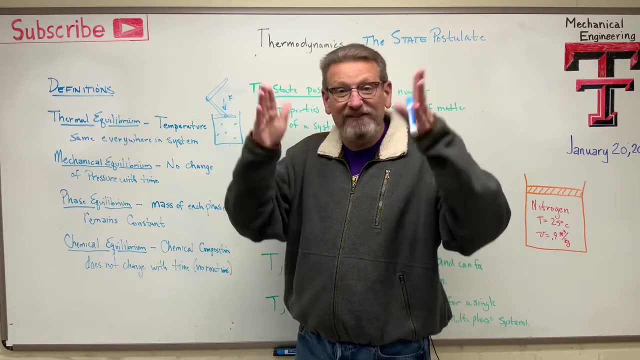 So if I had some kind of like a piston arrangement on here or something like that right, And it was putting some kind of downward force on my system in order to have mechanical equilibrium, I can't have a change in pressure there, I can't be squeezing on that or think I'd be still and normalized, equalized for us to have. 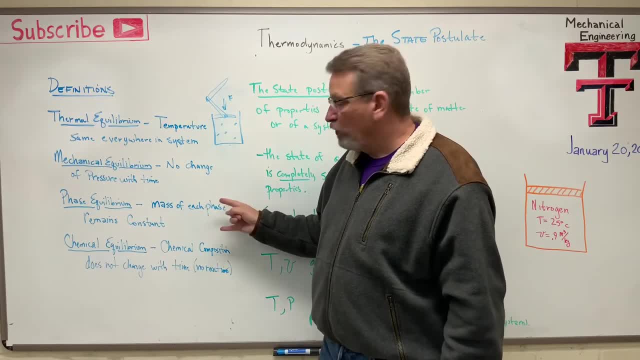 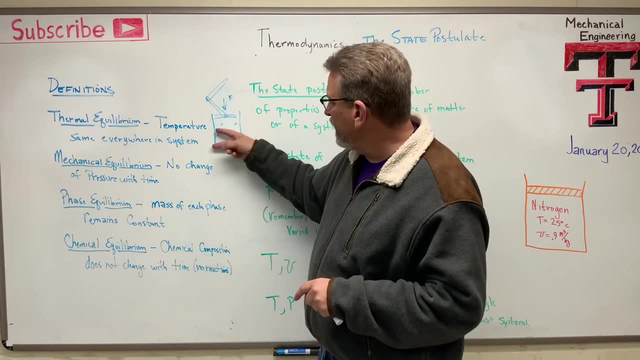 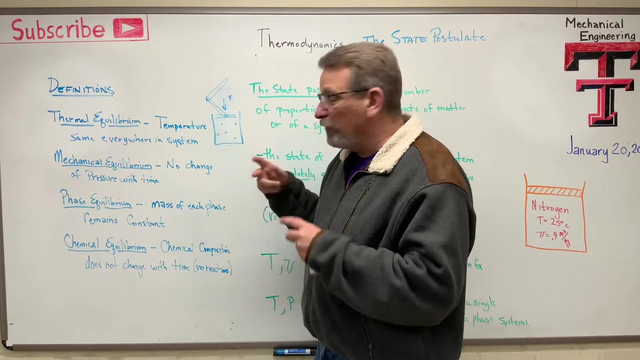 equilibrium, Phase equilibrium. okay, Remember your phases: solids, liquids, gases. right, The mass of each phase must remain constant. So you've got like if you had like a liquid like water in the bottom and then you had a gas over the top of that, maybe just air or something, then those have. 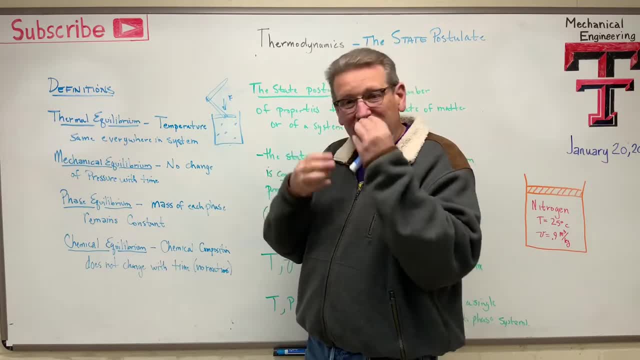 to be constant. So if you had a gas over the top of that, maybe just air or something, then those have to be constant. They have to be the same. They can't. there can't be any chemical reactions where they're changing. 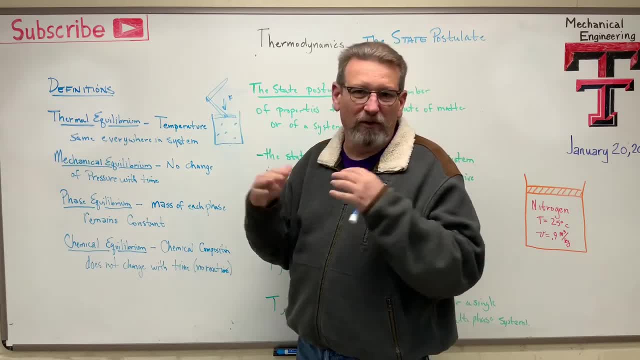 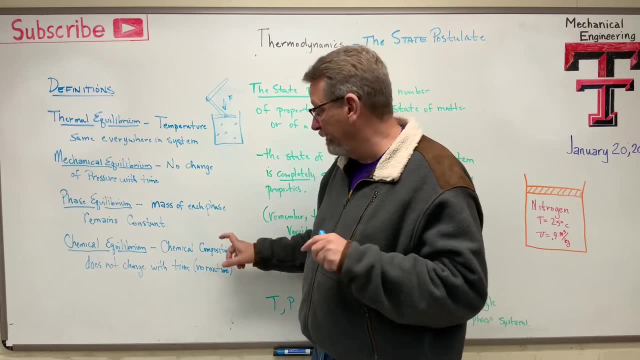 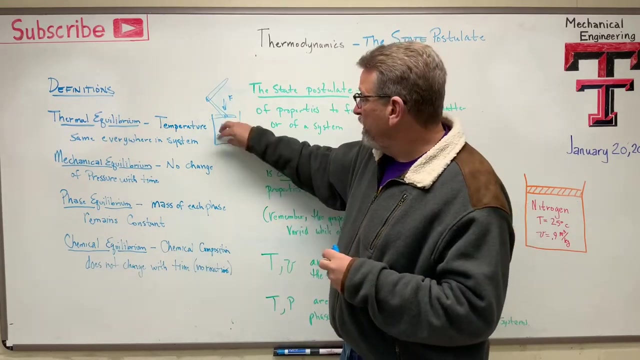 phases, or one's going to the other, a solid's going to a liquid or vice versa. So you have a phase equilibrium. when we look at, when we talk about state of equilibrium, We also have a chemical equilibrium, which means the chemical composition is not changing with time. So there's no chemical 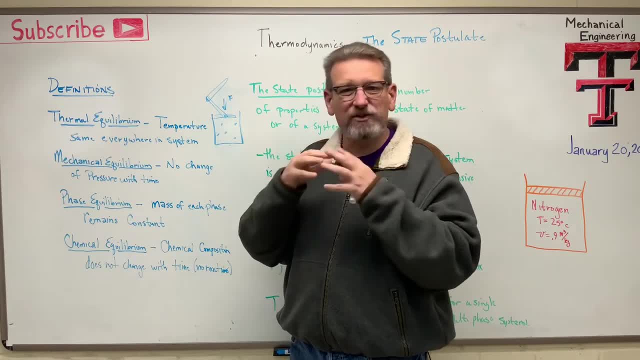 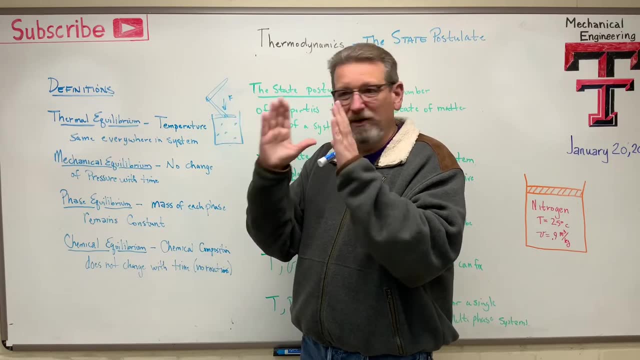 reactions in there. Those things aren't dissolving and giving off exothermic heat and doing all kinds of things. All that is done and it's just it's sitting there just like a glass of water. And if I come back tomorrow, 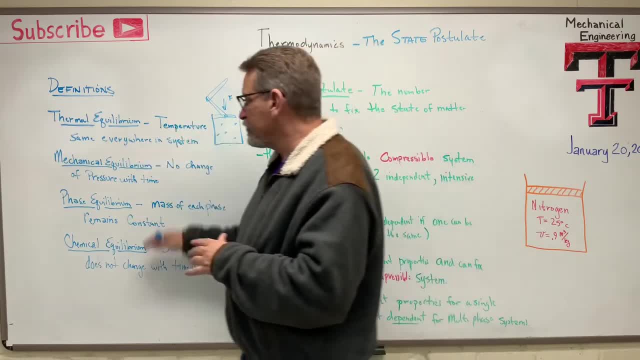 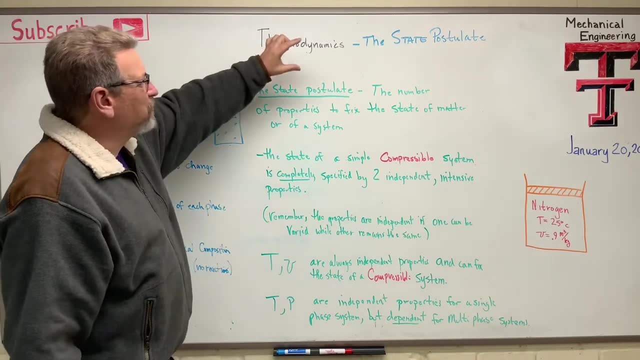 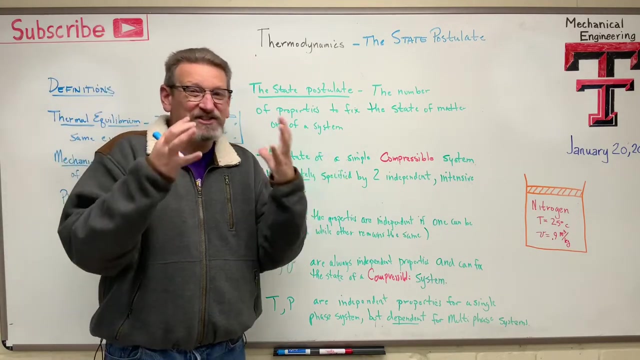 it's going to be the same exact composition tomorrow. Okay, So that's what we mean when we're talking about equilibrium of the system. Okay, So let's talk about the state postulate. Okay Now, the state postulate has to do with the state of the matter, the state of the system. 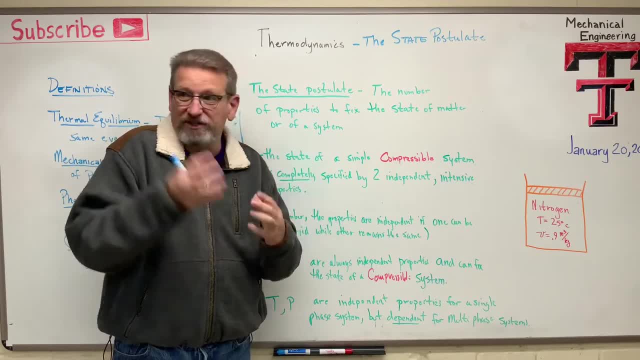 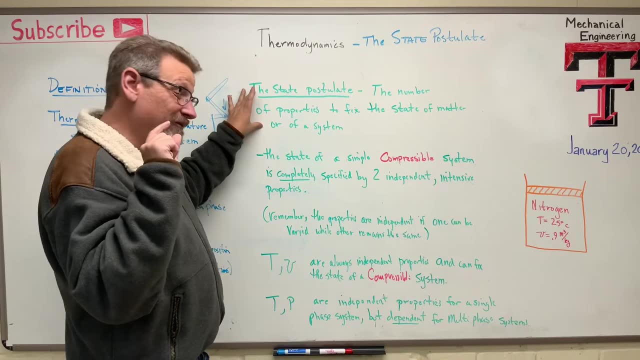 What's it doing, What's it feeling? What's the temperature, What's the pressure, What's the mass, What's the? you know all those things. right, Let's talk about the state. postulate that this is going to. this is going to be defining some 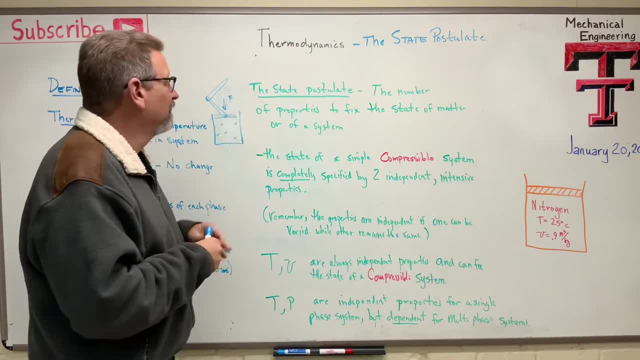 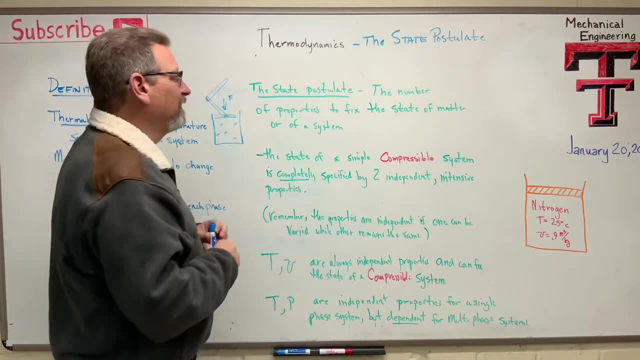 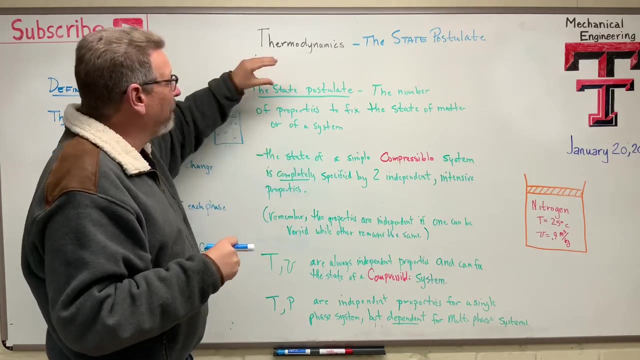 terms that tell us about the condition of the state of our system. So the number of properties to fix the state of matter or of a system is the state postulate. So how many things, the pressure, the temperature, the time or whatever it is- how many properties do I have? 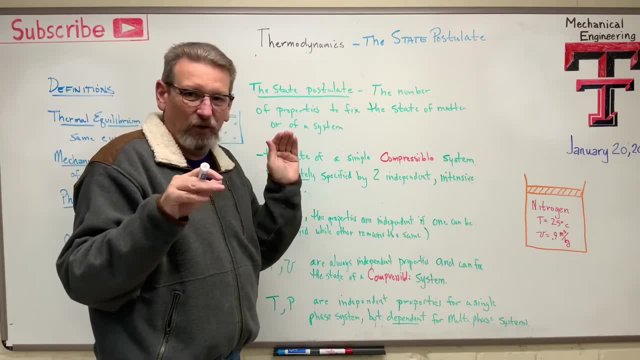 to have to fix the state of the matter so that I know everything there is to know about it. Okay, So here we go. Here's a little definition for us. This is important. This is probably a good one for thermo that you need to write this one down. 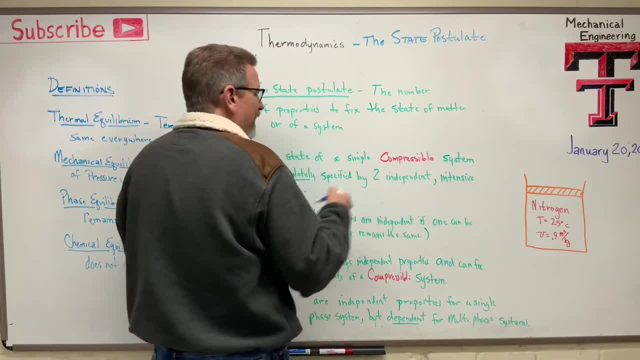 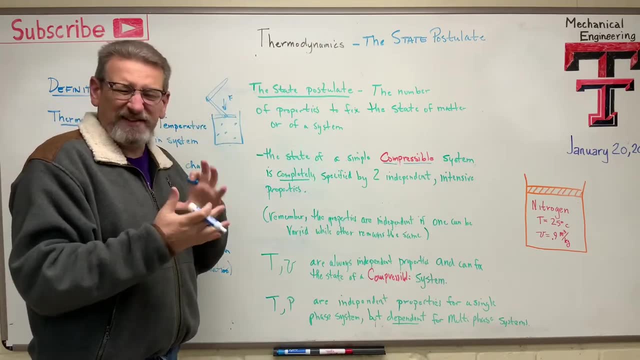 The state of a simple compressible. Now I've made that in red, I'm going to underline it right: Compressible system. This isn't an incompressible, but compressible system, which means it's some kind of gas, right, Or steam or something like that, right. 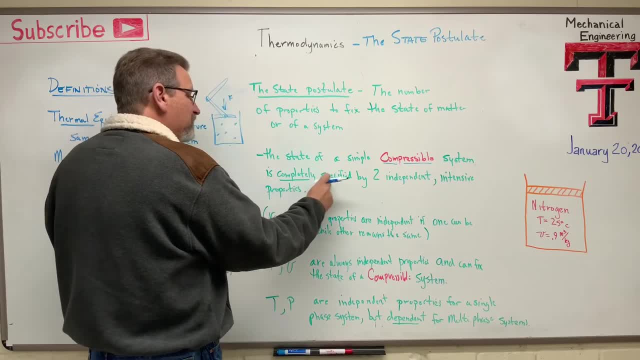 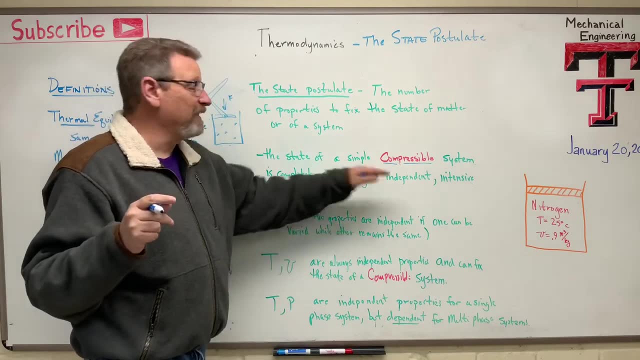 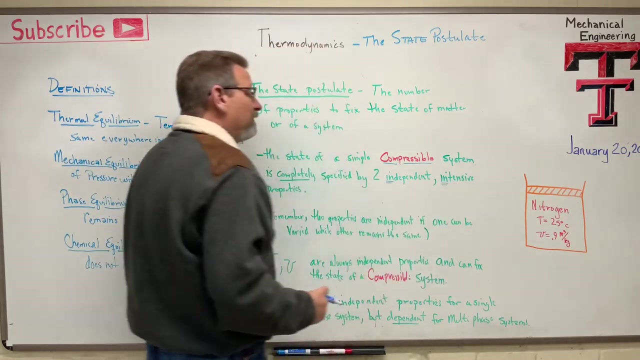 A compressible system is completely specified by two independent intensive properties And we, if you don't remember what intensive or independent properties are the last video, review that and remember this right. And dependent and intensive right, Those are properties that are not. they don't change if the size of the system changes. Okay, 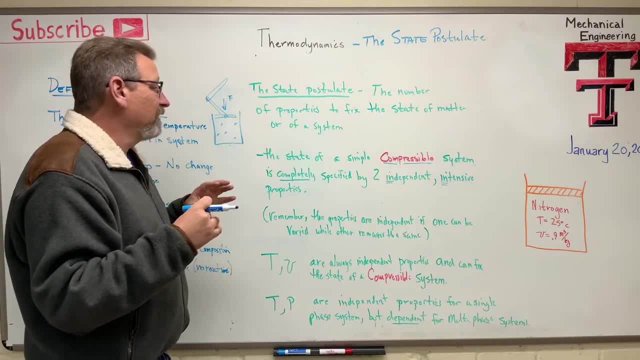 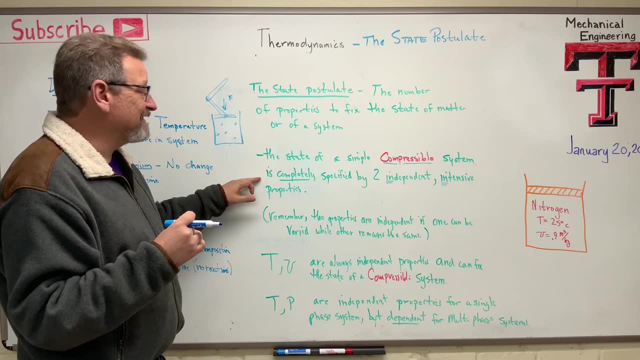 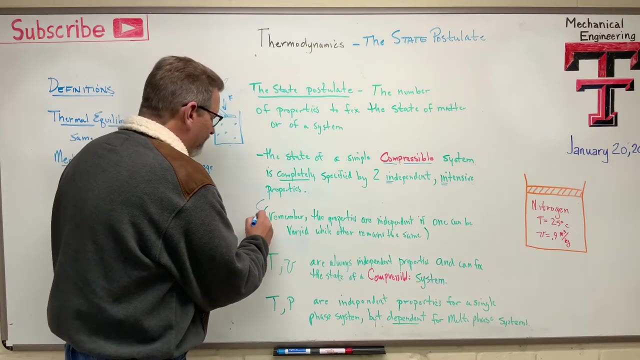 They don't change those properties. And so compressible system completely defined by two independent intensive properties. Okay, So here you go. Remember, the properties are independent. This is a little. this furthers our definition. Definition of an independent variable: Okay, Remember, the properties are independent If one. 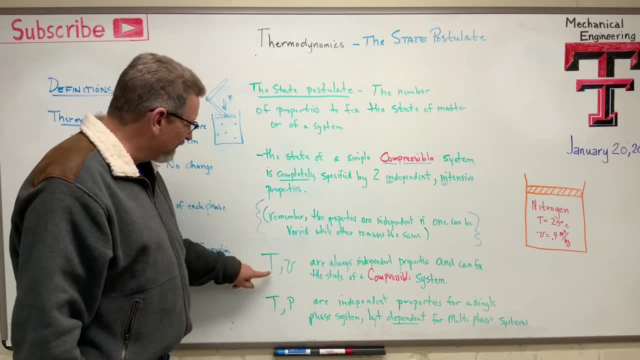 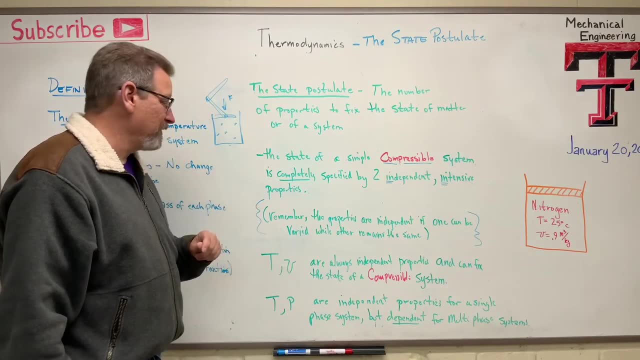 can be varied, while the other one stays the same. So if I have something like temperature and specific volume, if I change this one, that one doesn't change. That makes it an independent variable. Okay, So let's here's a couple more points here, kind of specific points that really. 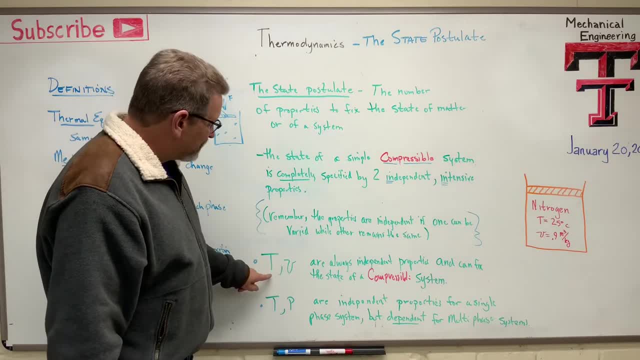 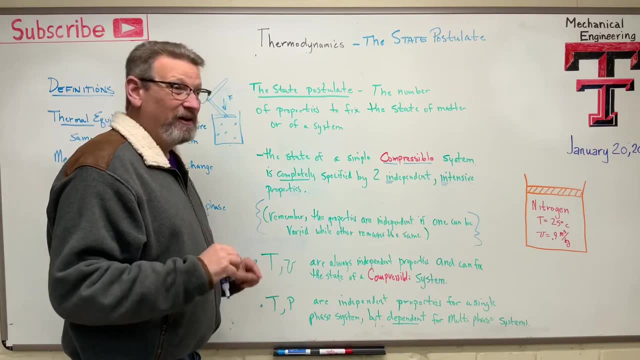 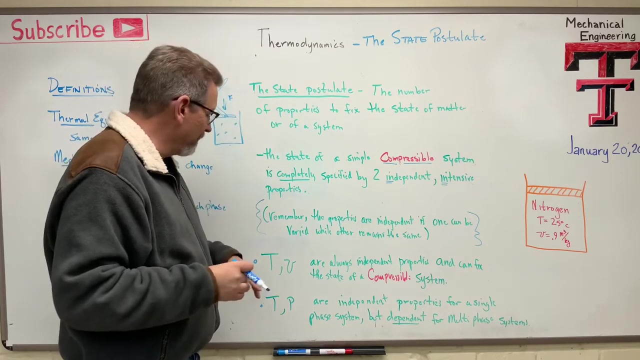 further define our system here. So temperature and what's little v? Do you remember we did that last video? That's specific volume. In other words it's like a per unit volume. What's the mass per unit of a little volume of whatever I have in my system? Remember, the volume of the whole system is. 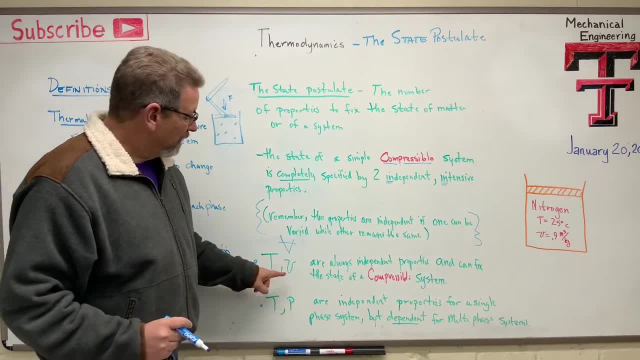 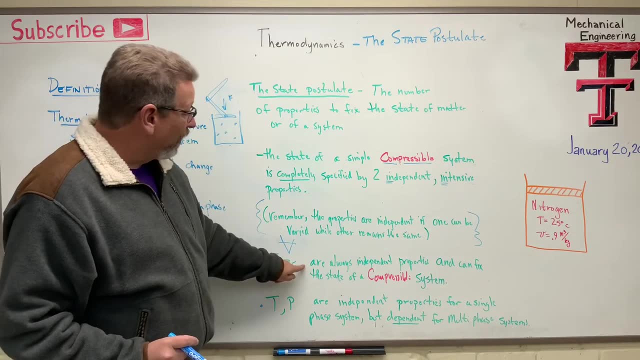 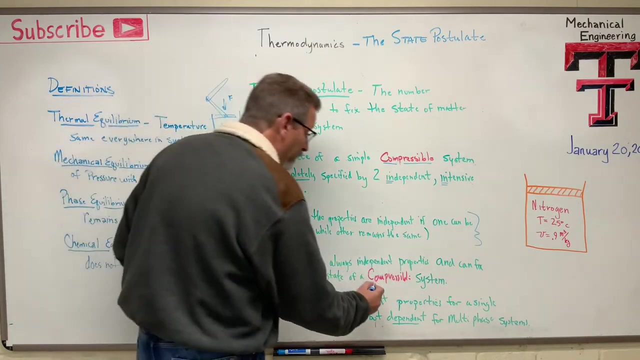 defined as this guy. We call him just big V, right, But little v is the specific volume. It's a per unit volume. So temperature and specific volume are always independent properties and can fix the state of a compressible system. Okay, Again, there we go with compressible again. Okay, So if I have generally for a compressible, 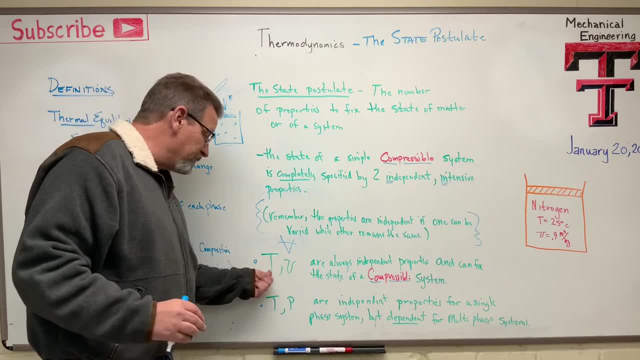 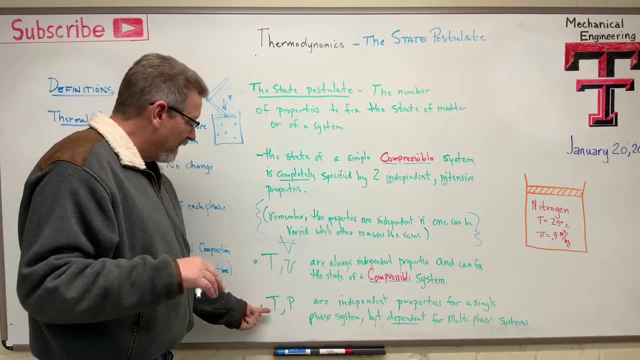 system, you're going to be given the temperature and the specific volume, Okay, And then we'll be able to tell everything else about the system. I'll show you an example right over here in just a second. So T and P- temperature and pressure- are independent properties for a single phase system. 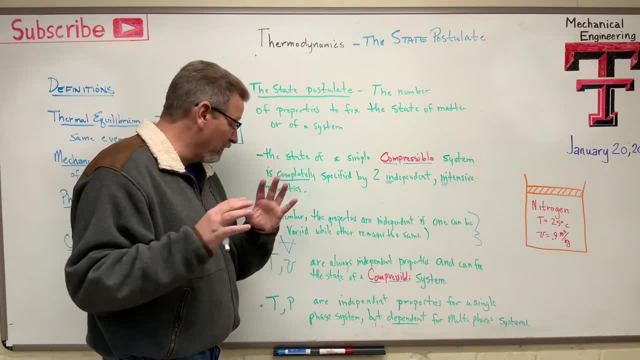 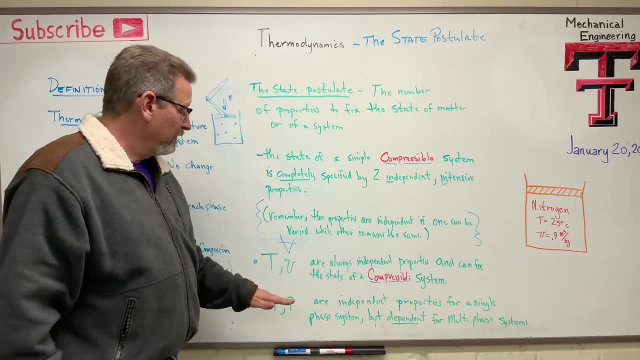 Like if the whole system was gas or the whole system was a liquid or whatever. right, But they're dependent for a multi-phase system. So if I have a single phase system, I'm going to have a multi-phase system. So once I mix the phases, these are not independent anymore. Okay, So that's. 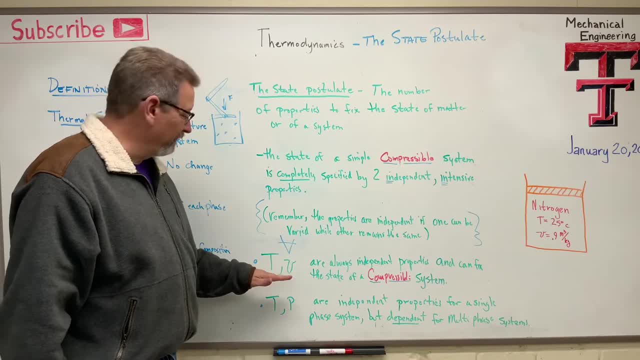 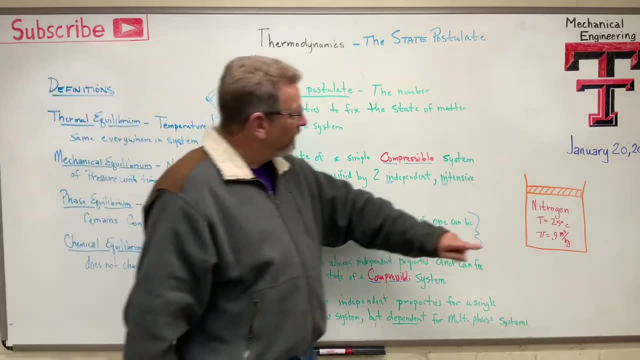 an important thing to remember. I know it's a lot to remember, isn't it? We'll try and make some rules up as we go along to help you remember, though. So temperature and specific volume. So let's look at this system. over here, Here's a system. What is the state of that system? Well, 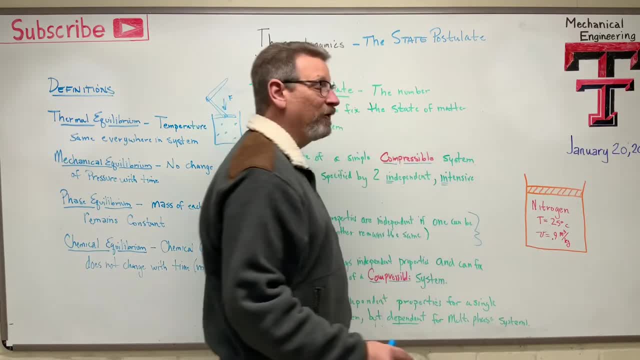 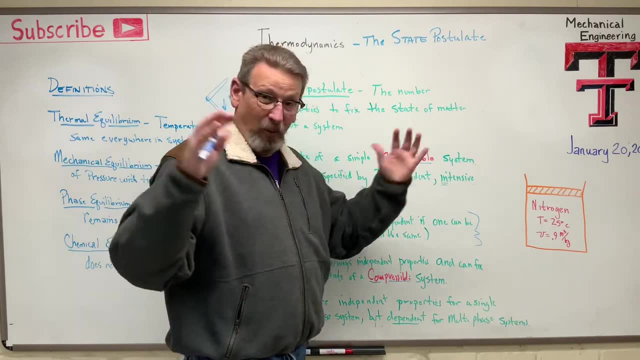 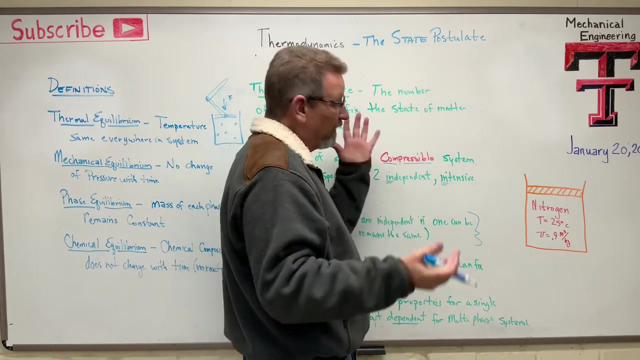 they tell us the temperature is 25 degrees C and the specific volume is 0.9 cubic meters. per kilogram of nitrogen takes up 0.9 cubic meters of volume. Okay, Add another cubic, add another kilogram, get another 0.9 cubic meters. right, That's what I mean. That's that's, that's specific.